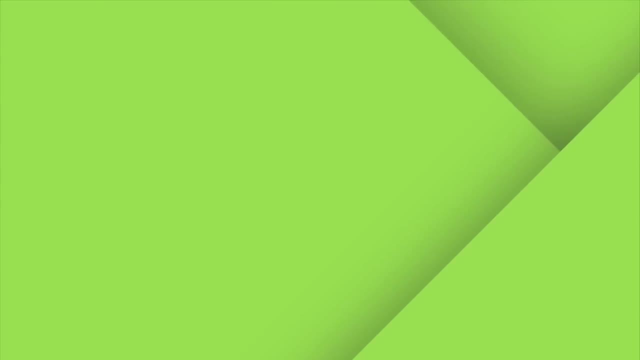 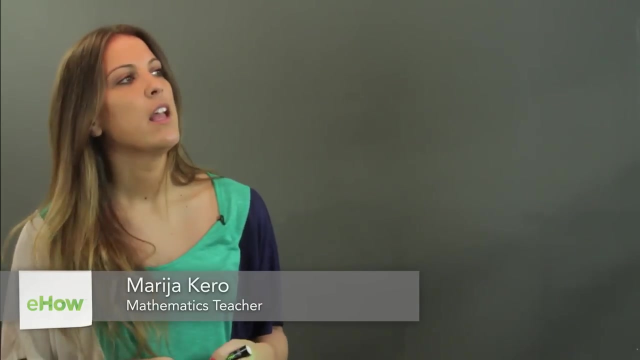 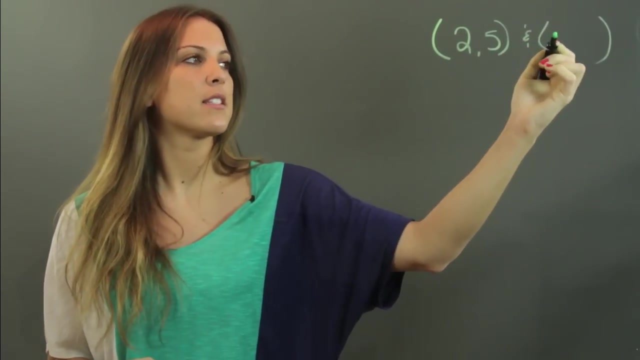 Hi, my name is Maria, I'm a mathematician and today I'm going to show you how to write a linear equation when you're given two points. So if I'm asked to write the equation of a line that goes through the points 2,, 5, and let's say 4, 9.. 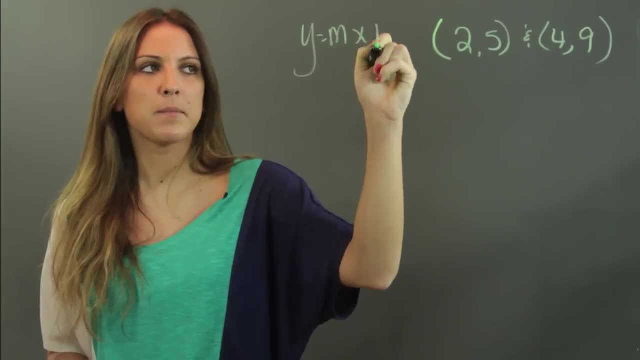 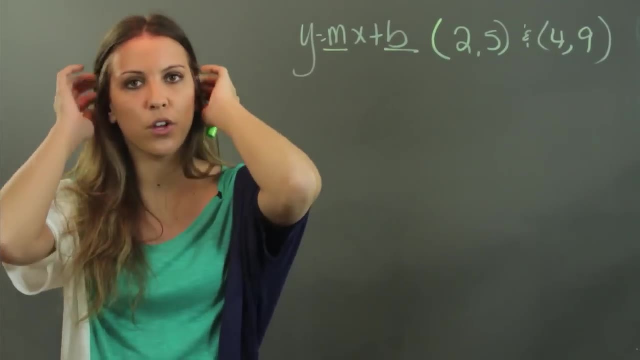 The first thing you should write down when you're asked to write an equation is: y equals mx plus b, the slope-intercept form of a linear equation, And what you need to know is that m and b are going to have to get filled in in order for your equation to be complete. 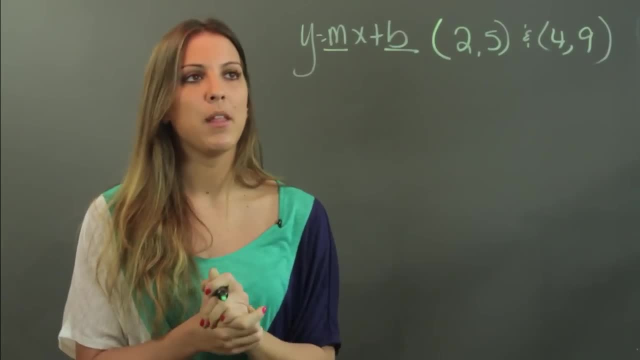 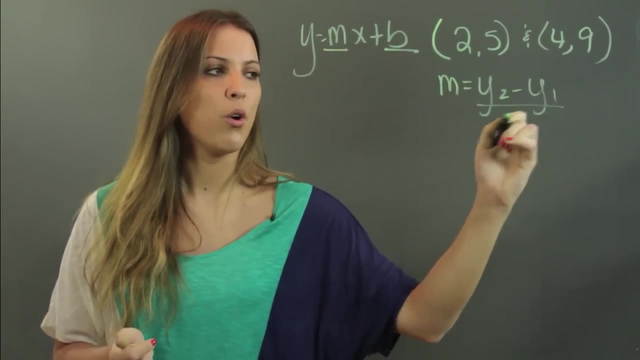 So now you have to ask yourself: how do you find m and how do you find b? Well, m is your slope, so you have to know the slope formula, which is: m equals y2 minus y1 over x2 minus x1.. 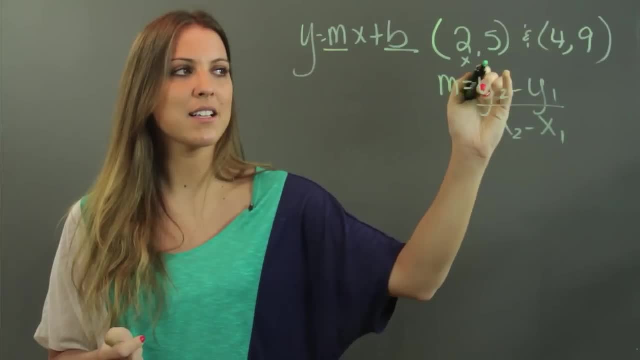 I'm going to go ahead and label these points and I know that every ordered pair has an x and a y, x and a y And I'm going to call this pair right here my 1, so that'll be x1, y1.. 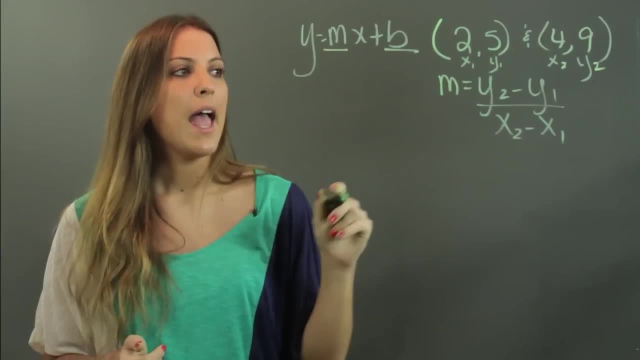 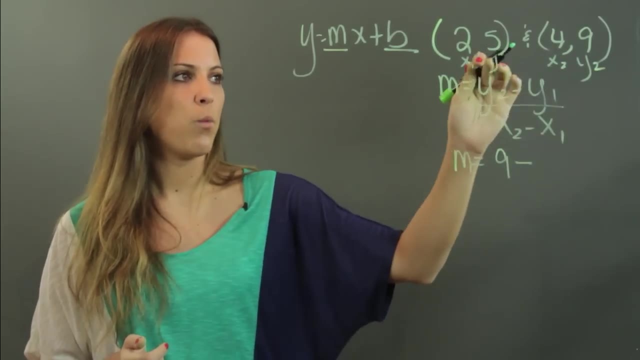 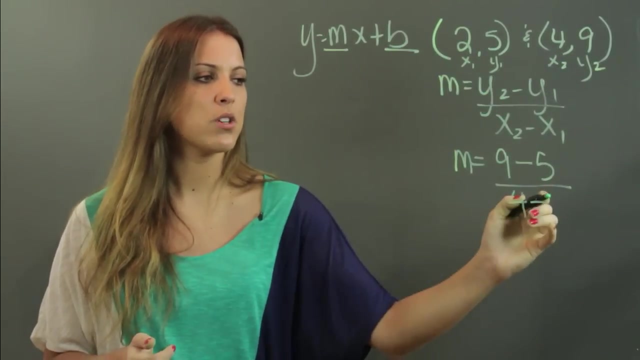 And this pair right here will be my 2.. So I get my 2s: x2,, y2.. And now I'm just going to substitute, So I get m equals y2, which is 9,, minus y1, which is 5,, over x2, which is 4, minus x1, which is 2.. 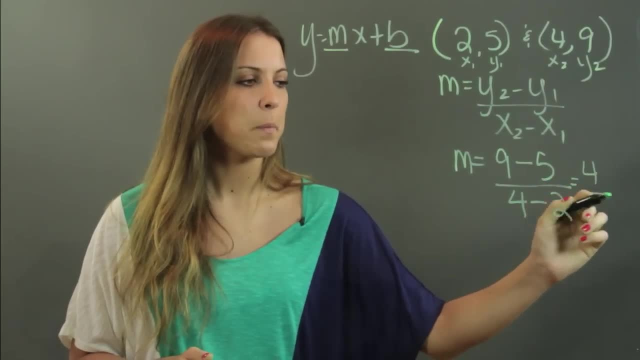 And now I'm going to go ahead and simplify: 9 minus 5 is 4,, 4 minus 2 is 2, and 4 divided by 2 is just 2.. So I found my slope. My slope is 2.. 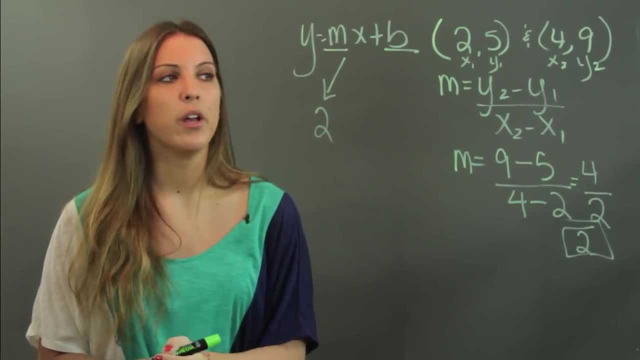 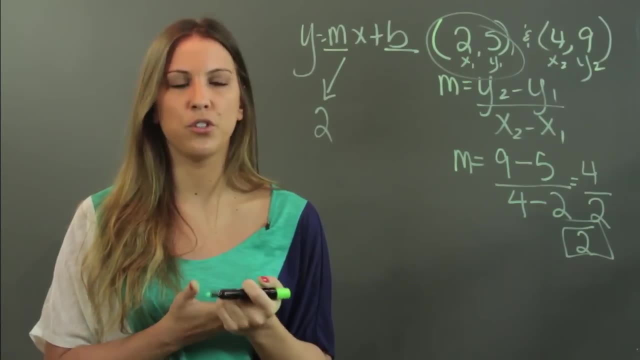 One part is done. Now to find b. Here's what you do. You pick whichever point you want, So I'm going to go ahead and pick this one, And it doesn't matter. so pick the one with the smaller numbers if that's easier for you to do. 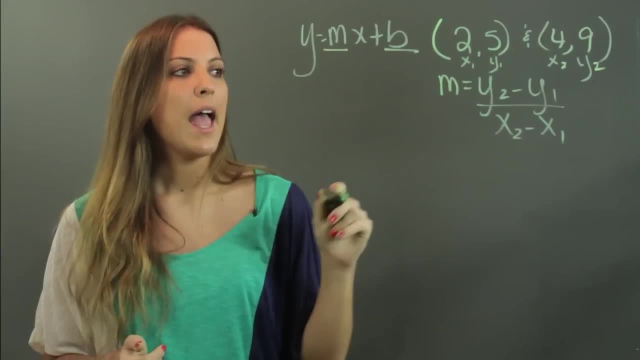 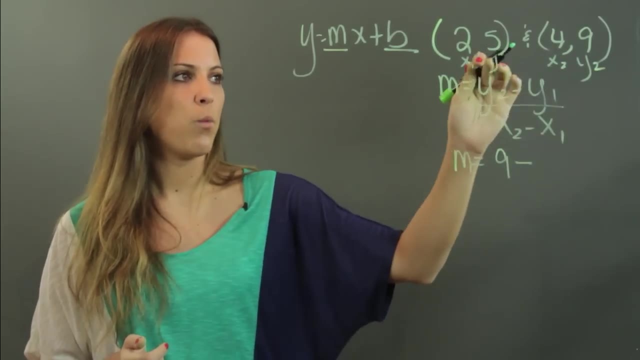 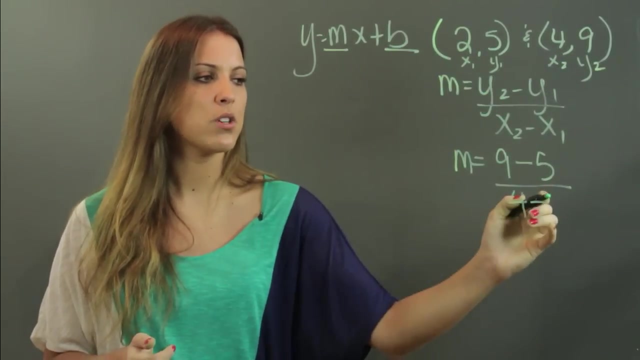 And this pair right here will be my 2.. So I get my 2s: x2,, y2.. And now I'm just going to substitute, So I get m equals y2, which is 9,, minus y1, which is 5,, over x2, which is 4, minus x1, which is 2.. 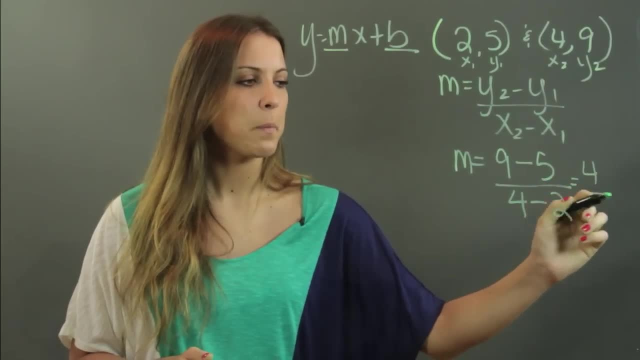 And now I'm going to go ahead and simplify: 9 minus 5 is 4,, 4 minus 2 is 2, and 4 divided by 2 is just 2.. So I found my slope. My slope is 2.. 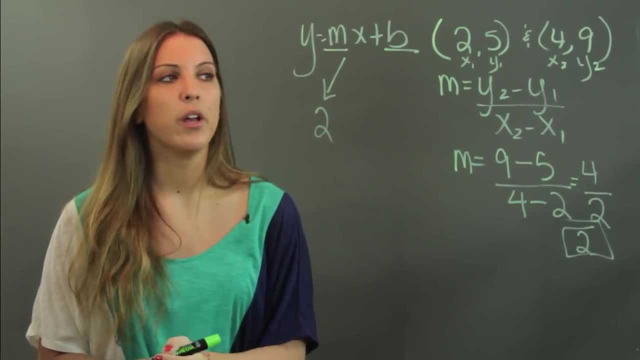 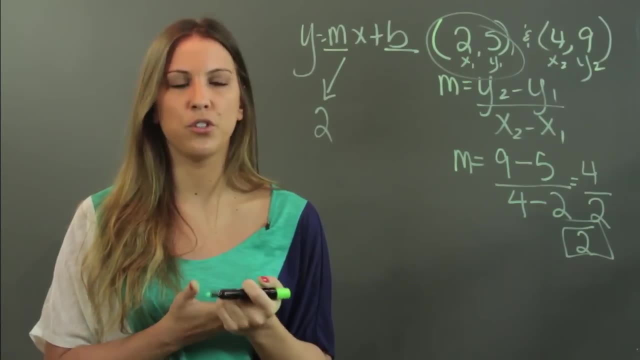 One part is done. Now to find b. Here's what you do. You pick whichever point you want, So I'm going to go ahead and pick this one, And it doesn't matter. so pick the one with the smaller numbers if that's easier for you to do. 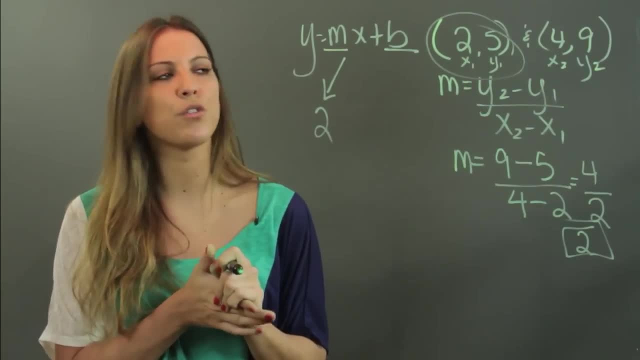 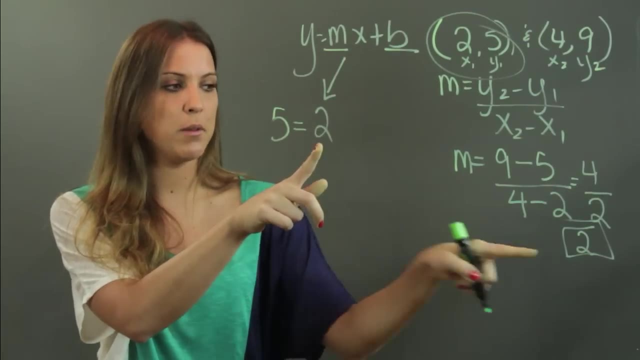 If I had one with negatives, avoid it and pick the positive one, because it's easier for you. And now I'm going to substitute y with 5.. I've already substituted my m with 2, because I solved for it. I'm going to substitute x with 2.. 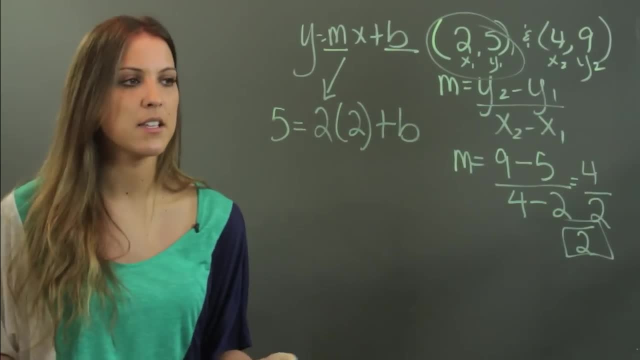 And I'm not going to substitute b with anything, because I'm trying to find out what b is. And now I just have to solve the equation: 2 times 2 is 4.. I'm going to get 4.. 5 equals 4 plus b. 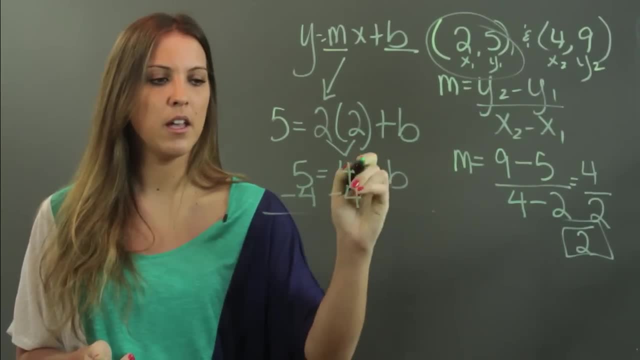 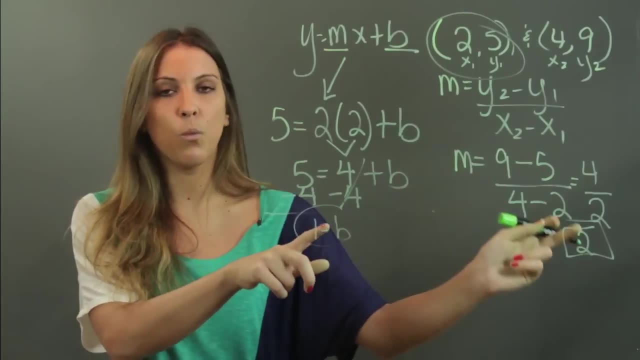 I'm going to use inverse operations and subtract 4 on each side to solve for b, And when I do that, I'm going to get 1 equals b. Now I've got the two vital parts of an equation, so I'm going to go ahead and rewrite it with these two parts in it. 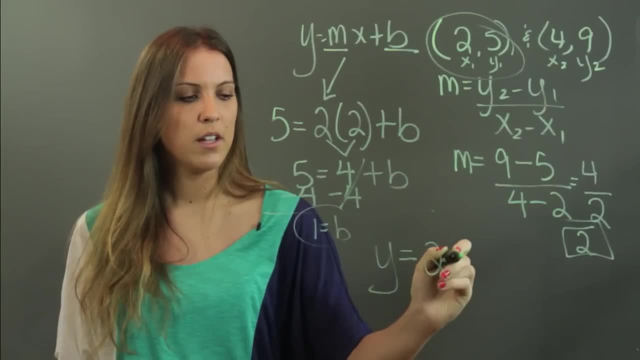 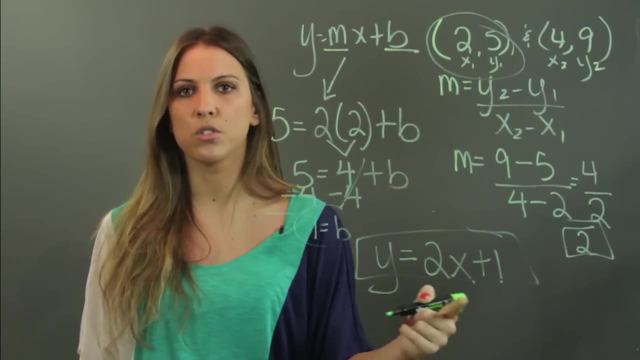 So I'm going to have y equals. instead of writing m, I'm writing 2x, And instead of writing b, I'm writing plus 1.. So the equation of the line that goes through these two points is: y equals 2x plus 1.. 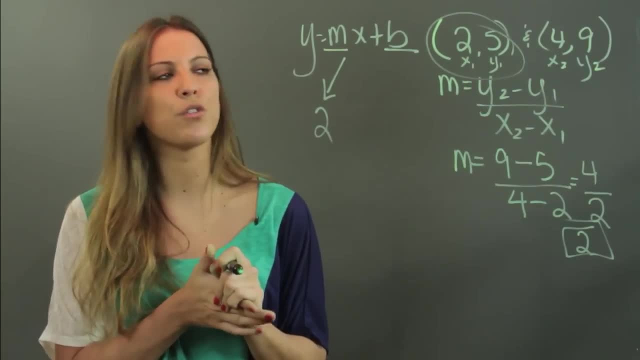 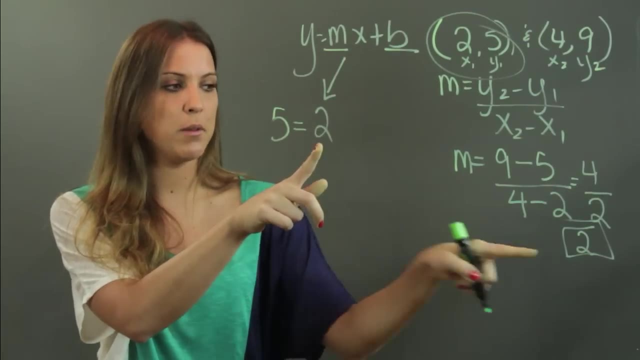 If I had one with negatives, avoid it and pick the positive one, because it's easier for you. And now I'm going to substitute y with 5.. I've already substituted my m with 2, because I solved for it. I'm going to substitute x with 2.. 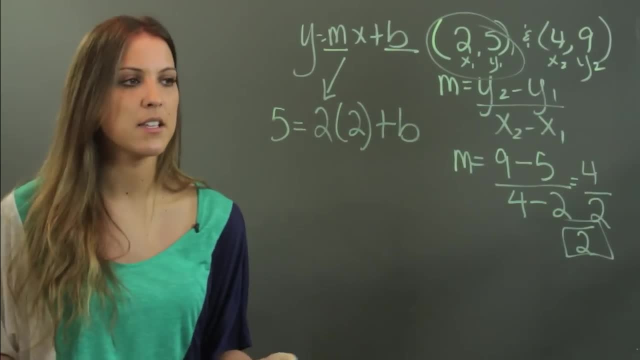 And I'm not going to substitute b with anything, because I'm trying to find out what b is. And now I just have to solve the equation: 2 times 2 is 4.. I'm going to get 4.. 5 equals 4 plus b. 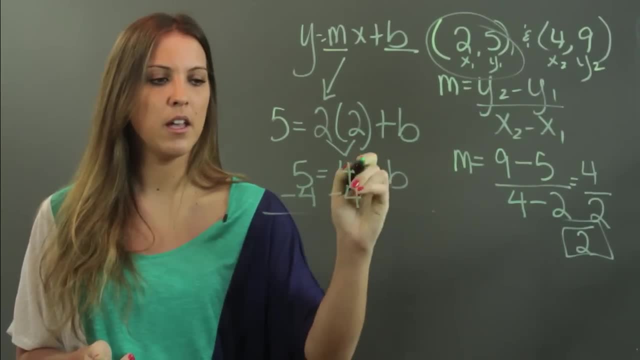 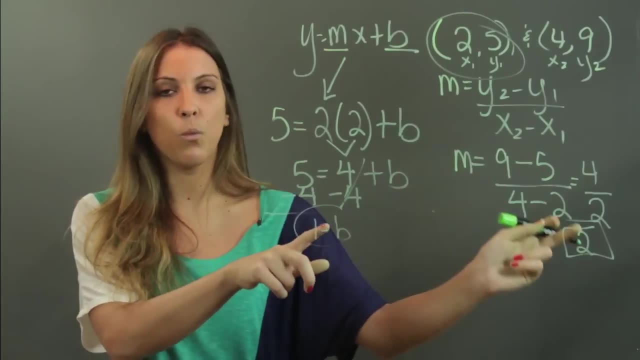 I'm going to use inverse operations and subtract 4 on each side to solve for b, And when I do that, I'm going to get 1 equals b. Now I've got the two vital parts of an equation, so I'm going to go ahead and rewrite it with these two parts in it.